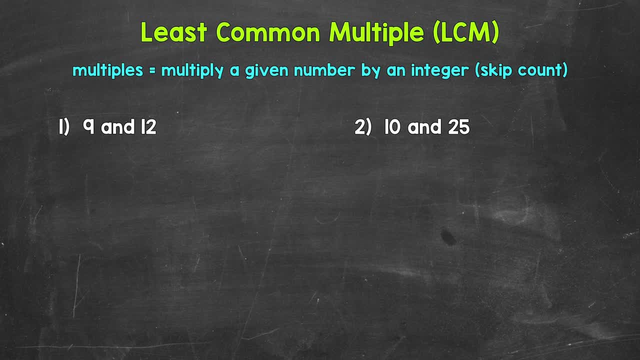 number by an integer. When we think of the multiples of a number, we need to think about the numbers we get when multiplying that given number by integers. A simpler way to think about multiples is to think about the numbers we get when multiplying that given number by integers. 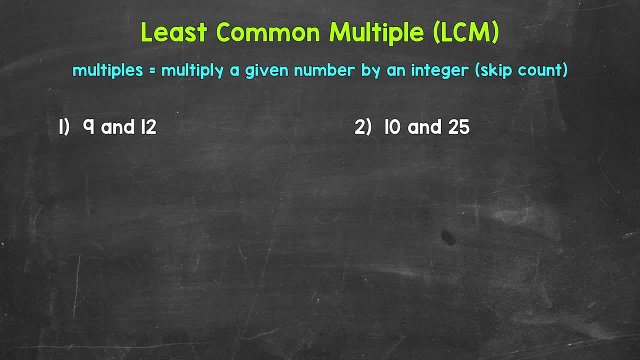 Think about skip counting. So all of the numbers, something is going to hit when you count up by that number. Those are all going to be multiples. This will make a lot more sense as we go through our examples. Let's jump into our examples, starting with number 1, where we have 9 and 12.. 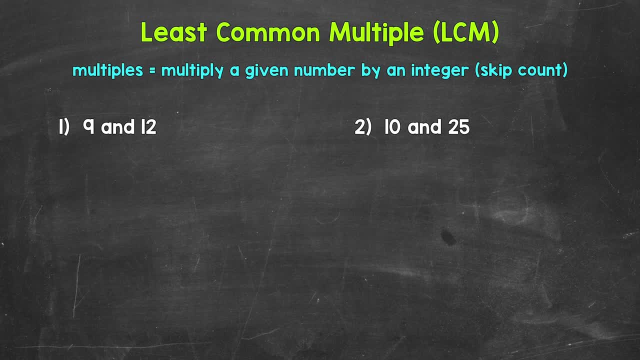 We're going to start by listing some multiples of both 9 and 12.. Then we will look for common and specifically the least common multiple, also referred to as the LCM. Let's start with some multiples of 9,, which are 9 times 1,, which is 9.. 9 times 2 is 18.. 9 times 3 is 27.. 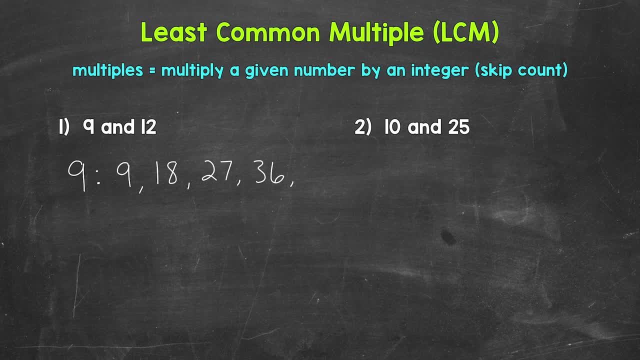 9 times 4 is 36. And 9 times 5 is 45. So you can see that we just skip counted by 9, to list those multiples: 9,, 18,, 27,, 36,, 45,, so on and so forth. Now I stopped at 45 because 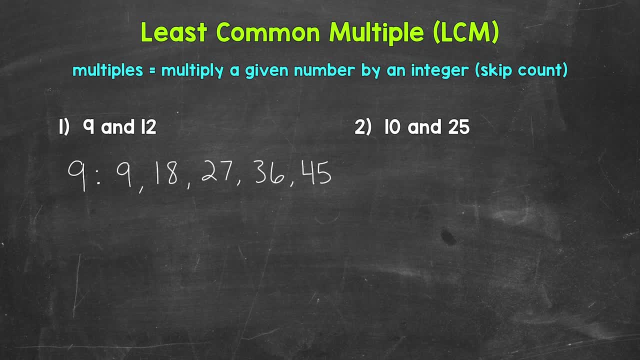 multiples go on forever. They are endless, They are infinite. My suggestion is to list 4 or 5 multiples when looking for the least common multiple. So list 4 or 5 multiples for each number, Look for any in common And if you don't have any in common, 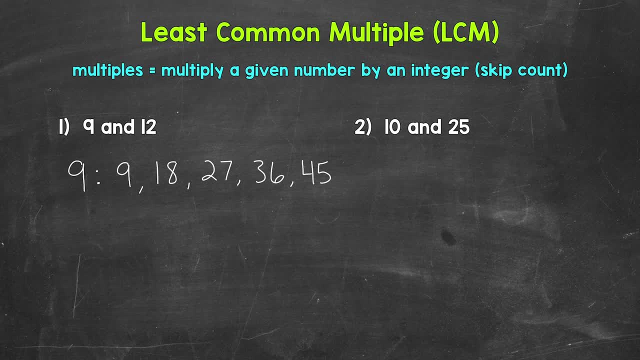 you can always extend the multiples lists. Now let's list the first 5 multiples of 12.. 12 times 1 is 12.. 12 times 2 is 24.. 12 times 3 is 36.. 12 times 4 is 48.. And 12 times 5 is 60.. 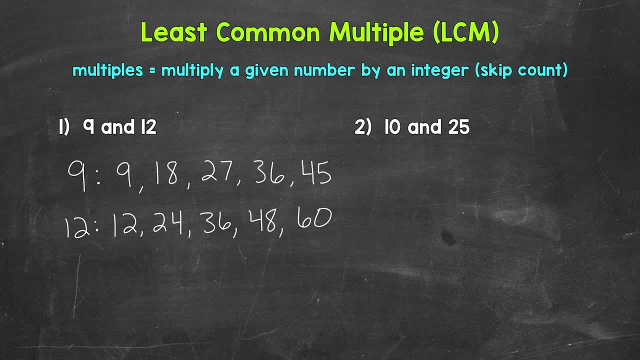 So again, you can see that we skip counted there. We skip counted by 12.. So 12,, 24,, 36,, 48,, 60, so on and so forth, Now that we have some multiples listed for both 9 and 12,. 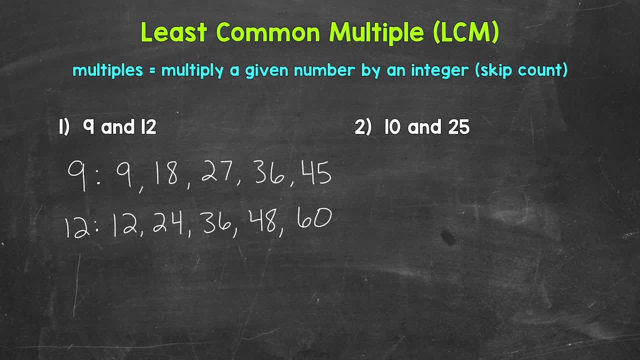 we need to look for any common multiples, So any multiples that they share, And then, specifically, we need to look for the least common multiple. Well, 36 is a common multiple And it's going to be the least common multiple, So the smallest. 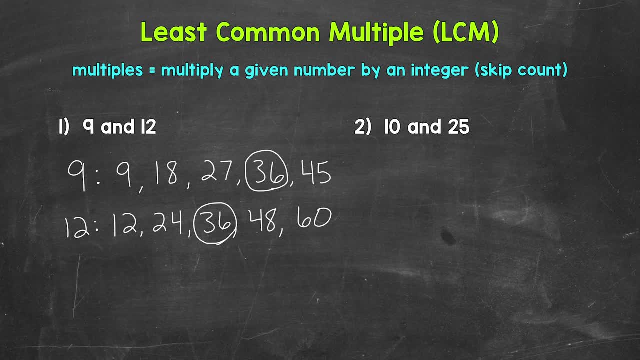 multiple in value that they share. So let's write that the LCM, which stands for least common multiple, is 36.. So the least common multiple of 9 and 12 is 36.. Now, one thing I do want to mention about common multiples is that they are infinite, Although we only have one common multiple in our 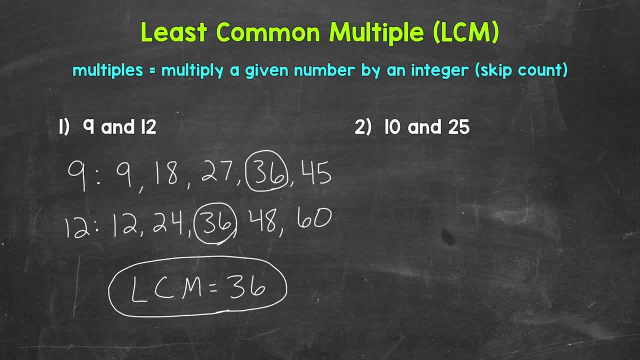 lists, as is 36, we can always extend multiples, So let's look for any common multiples that they share. So let's take a look at the list of lists So we can always keep going to find more common multiples. Remember, multiples are endless, So that means common multiples are endless, So that's just. 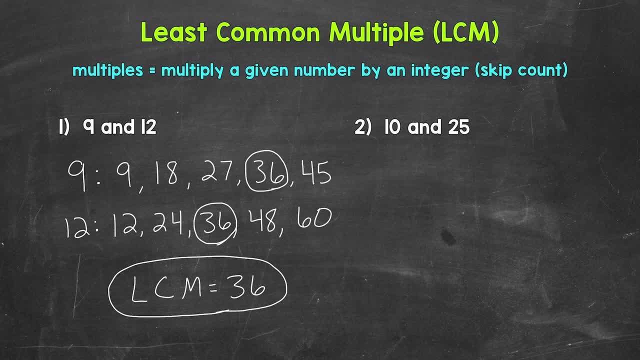 something to think about when it comes to multiples. Let's move on to number 2, where we have 10 and 25.. Let's start with some multiples of 10.. So 10 times 1 is 10.. 10 times 2 is 10.. 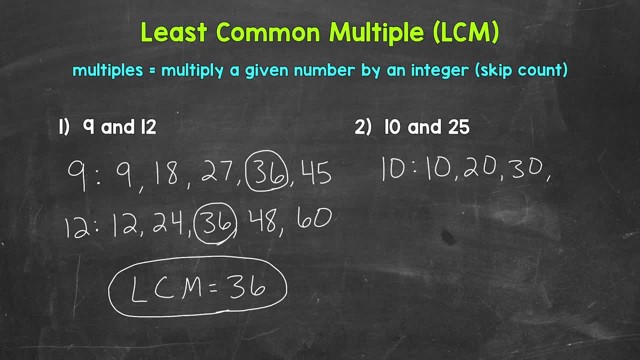 20,, 10 times 3 is 30,, 10 times 4 is 40,, and then 10 times 5 is 50. So 10,, 20,, 30,, 40,, 50,, so on, and 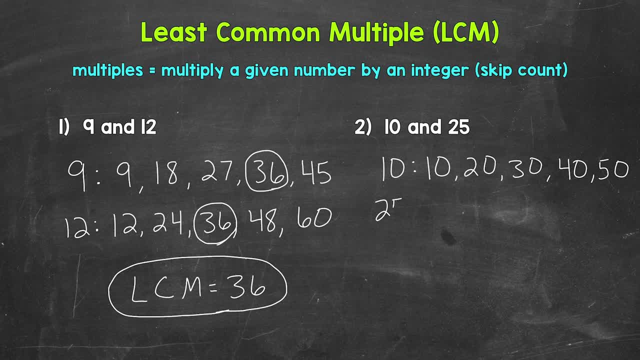 so forth. Now let's list the first five multiples of 25.. So 25 times 1 is 25, 25 times 2 is 50, 25 times 3 is 75, 25 times 4 is 100, and then 25 times 5 is 125.. Now that we have some multiples. 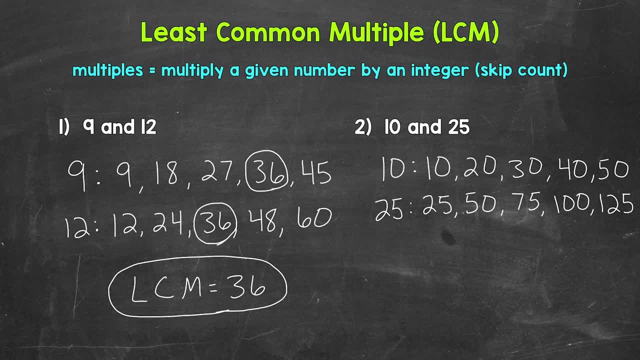 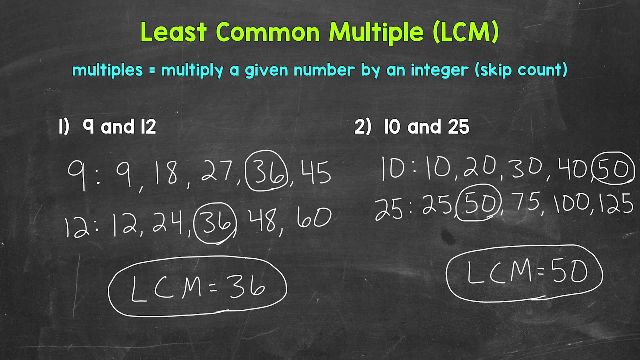 listed. we can look for common multiples and specifically the least common multiple. Well, 50 is a common multiple and it happens to be the least common multiple, So the LCM is 50.. 50. The least common multiple of 10 and 25 is 50.. So there's how we list out some multiples of. 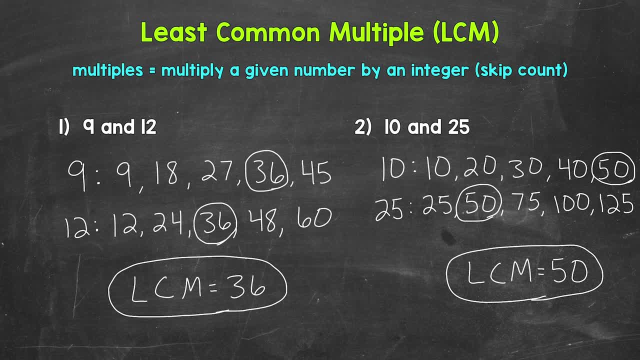 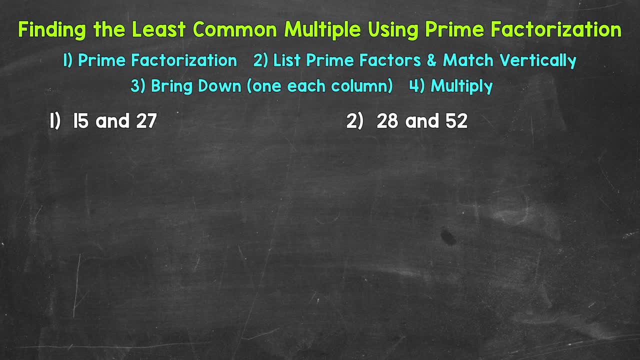 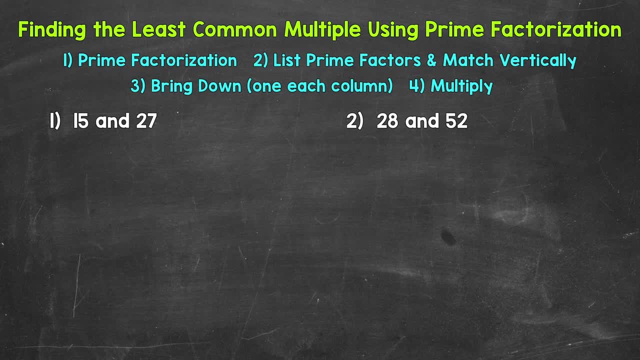 the most common. For example, the strategy of listing out multiples of numbers in order to find the LCM can be kind of difficult and time-consuming when working with. so this is a different approach, a different strategy to be familiar with when it comes to finding the. 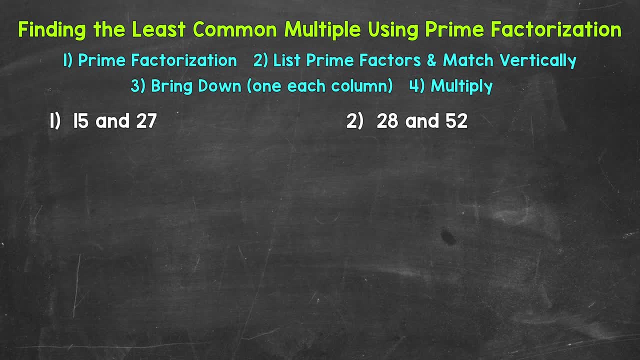 least common multiple. So let's Let's jump into our examples, starting with number one, where we have and 27.. Let's start with the prime factorization of 15, and we will start with the factors of 3 and 5.. Now, 3 is prime, so we are done there, and 5 is prime, so we are done there as well. 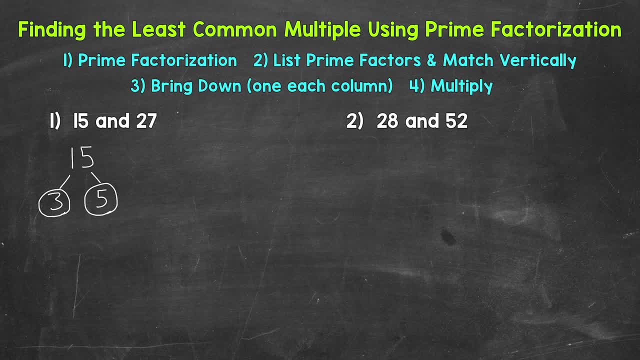 and that's the prime factorization of 15.. We can't break that down any further. Now we have the prime factorization of 27.. Let's start with the factors of 3 and 9.. 3 times 9 equals 27,, so 3 and 9 are factors of 27.. 3 is prime. so we are done there. 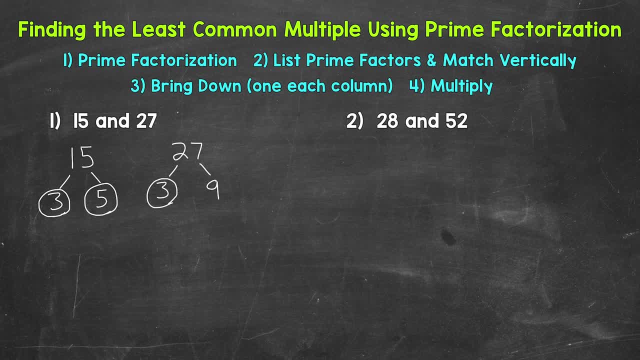 but we can break 9 down: 3 times 3 equals 9, so 3 is a factor of 9.. 3 is prime, so we are done there. and 5 is prime, so we are done there. So we are done there and there, And that's the prime factorization of 27.. We can't break that. 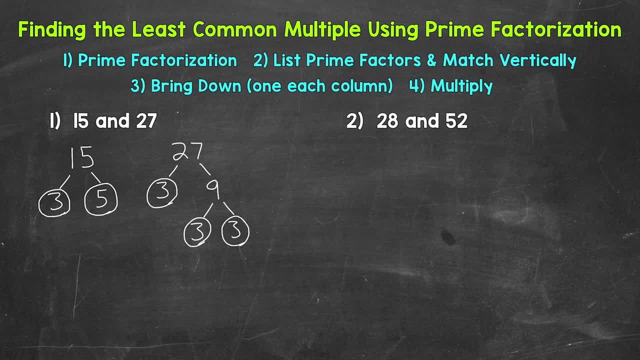 down any further. Now we're ready to move to the next step, So we need to list the prime factors of 15 and 27 and match them vertically. Let's see what this looks like, starting with 15.. So our prime factors from the prime factorization are 3,. 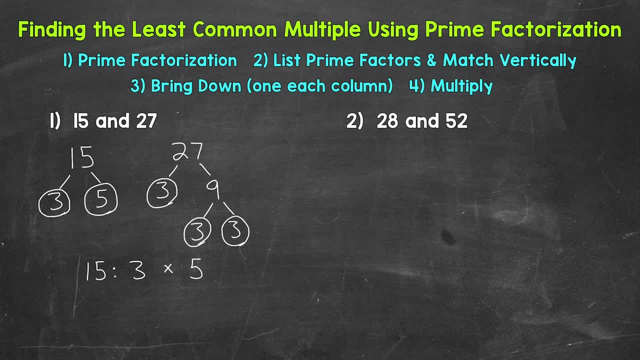 and 5, or 3 times 5.. Now 4, 27.. So we have 3 times 3 times 3, and you'll notice that big gap underneath the 5. there We are matching numbers vertically. 27 does not have a prime factor of 5,. 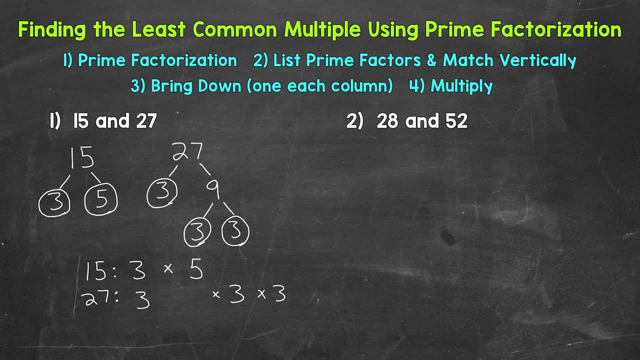 so I left that blank underneath the 5.. Now that we have our prime factors listed and matched vertically, we move on to the next step, where we bring down, And I like to draw a line underneath here in order to separate these steps. So this is a column. 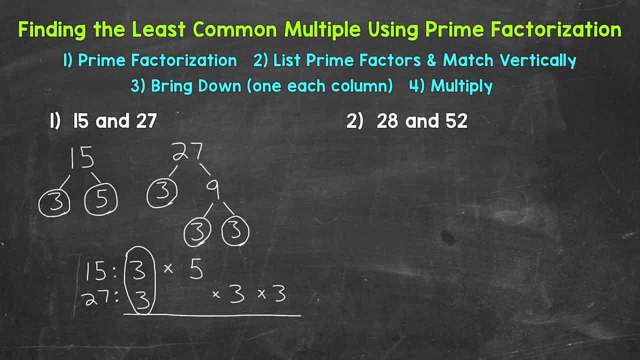 and although we have two 3s here, this is a column of 3s, So we just bring one down. We have a 3 to represent that column of two 3s times. we have a column of 5 here times. we have a 3 here times another 3 here. 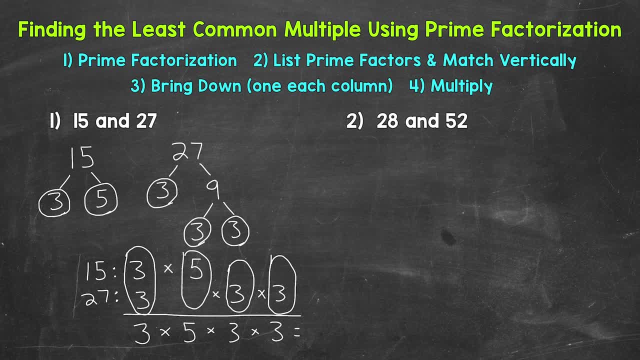 So we end up with 3 times 5 times 3 times 3.. And by multiplying these we get our least common multiple. So 3 times 5 is 15, times 3 is 45, times 3 is 15.. So we end up with 3 times 5 times 3 times 3.. 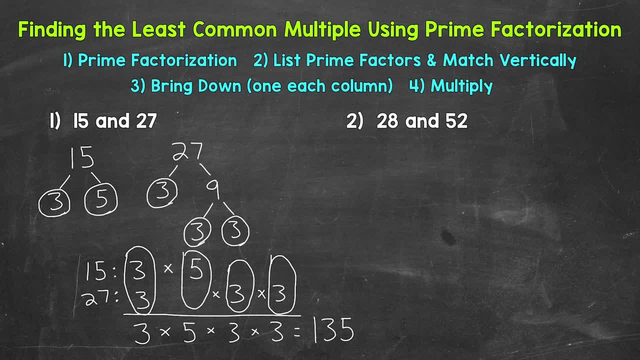 We start by multiplying these to nothing but 5.. And that's actually our least common multiple. And now, without doing this, when we check, we find that all of our same values have the sameATE. Therefore, we move onto line 3, and then we'll continue. This is going to me, Judith's. 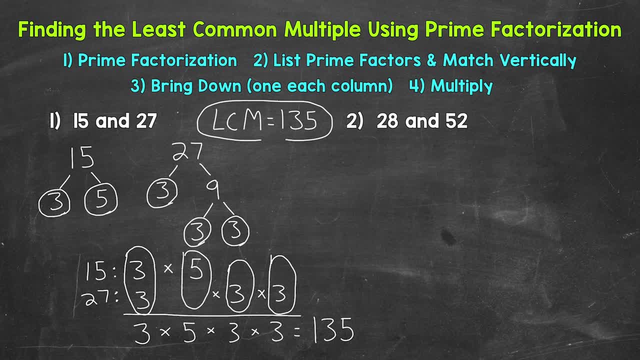 4s plus dry. So the following one is going to be 3s plus dry, The other two 5s and 5s. here we're going to draw onto the similar two lines of our start, which I just hope everyone will be able to do because there's so many numbers here. 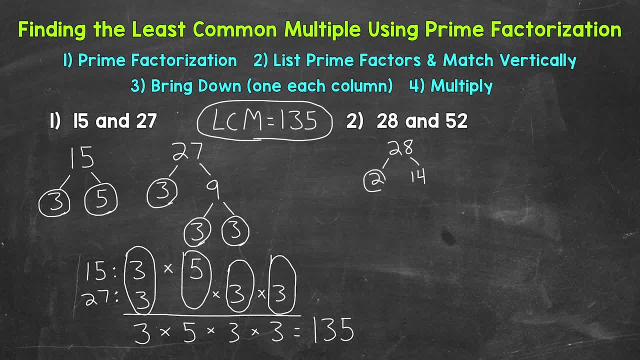 let's start with those factors. 2 is prime, so we are done there. 14, we can break down 2 times 7, equals 14, so 2 and 7 are factors of 14.. 2 is prime, so we are done there. 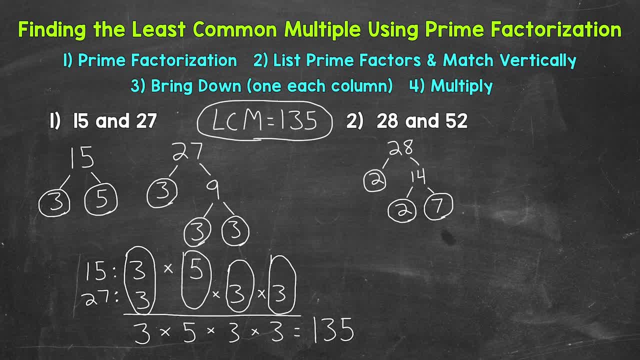 And 7 is prime as well. so we are done there, And that's the prime factorization of 28.. We can't break that down any further. Now we need the prime factorization of 52.. Let's start with the factors of 2 and 26.. 2 times 26 equals 52,, so 2 and 26 are factors of 52.. 2 is prime, so we are done. 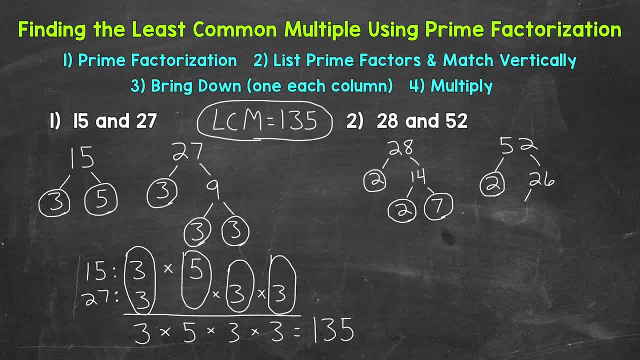 there 26. we can break that down: 2 times 13 equals 26,. so 2 and 13 are factors of 26.. 2 is prime, so we are done there, And 13 is prime as well, so we are done there, And that's. 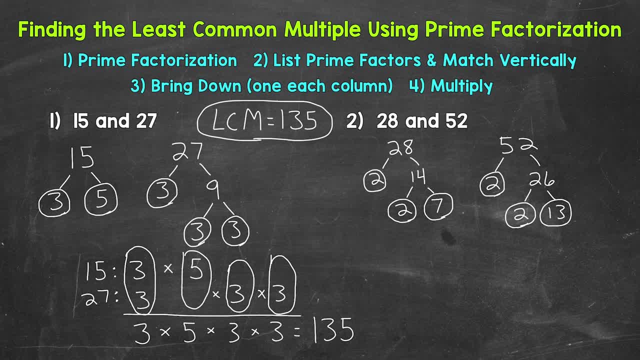 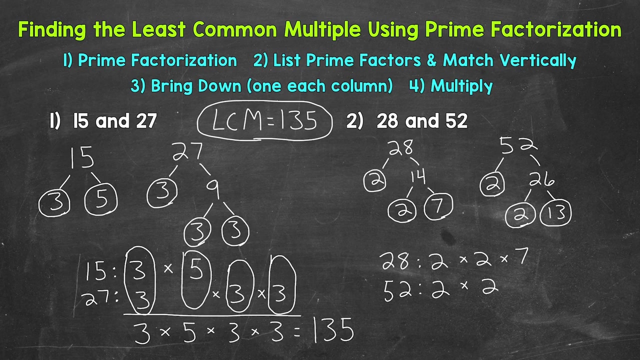 the prime factorization of 52.. We can't break that down any further. Now we need to list the prime factors and match them vertically: For 28, we have 2 times 2 times 7.. For 32,, we have 2 times 2 times 13.. Now we need to bring down. So we have a column. 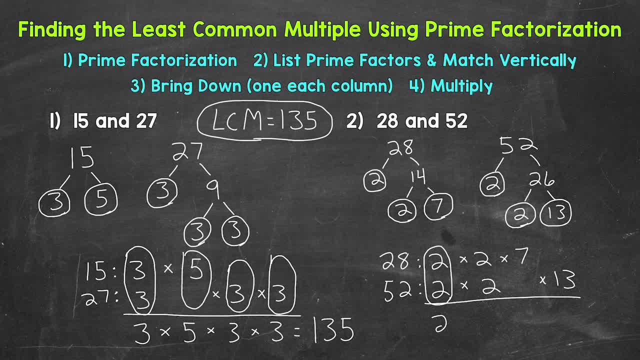 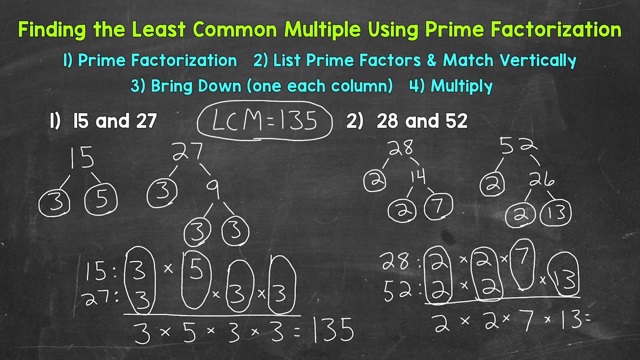 of 2s here. so let's bring down a 2 to represent that column times another column of 2s. So let's bring another 2 down times 7.. So we have 4 times 7 times 13.. So we have 2 times 2 times 7 times 13, to get our least common multiple. 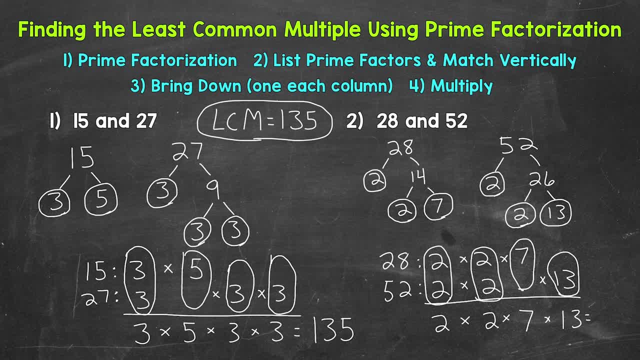 We have 2 times 2, which is 4.. Times 7 is 28 times 13.. Well, I'm not sure what 28 times 13 is, so let's come to the side here And multiply 28 times 13..